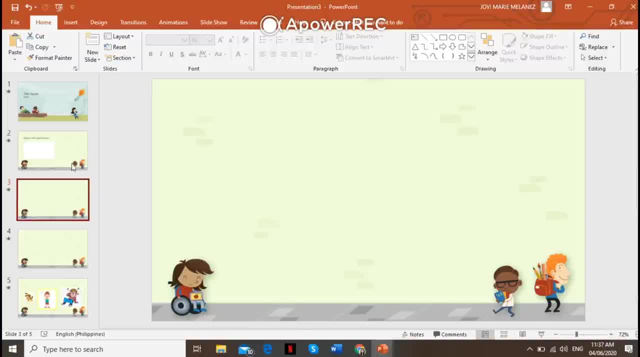 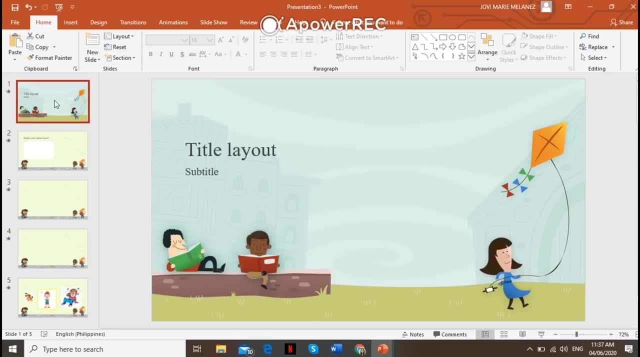 it will be linked to this slide. When they get the wrong answer, the slide will be linked to this slide. So let's start by putting our title: What is the beginning letter? So it's a game. They are going to click the beginning letter. 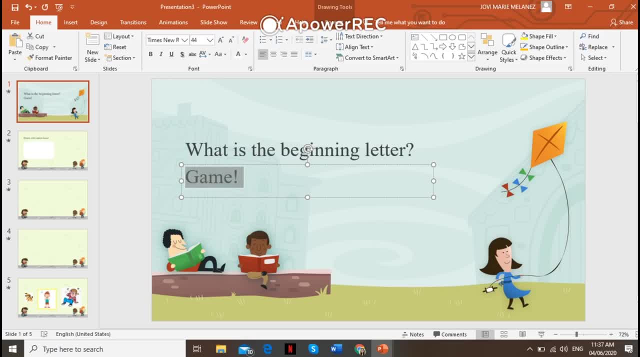 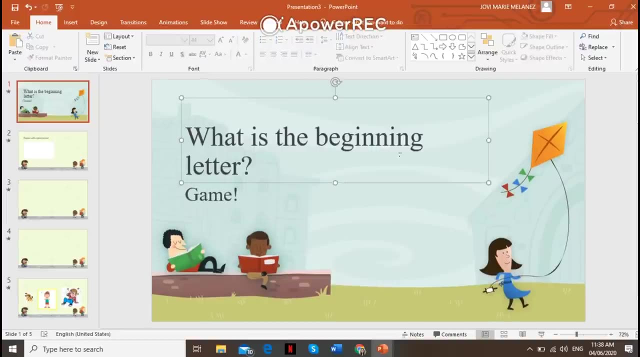 This is just an example. You can make your own. You can make another game that you want That is similar to this one. Okay, Let's make it bigger. We can layout it properly. You can change the color or whatever you want to do here. 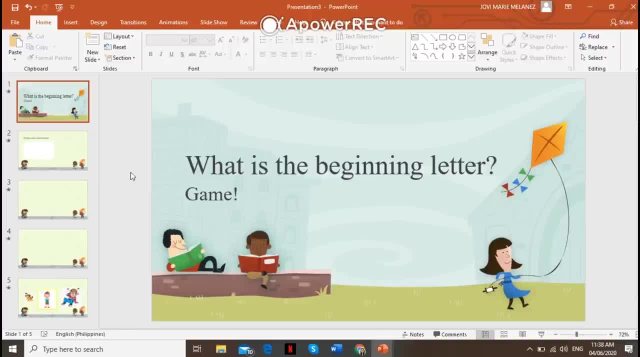 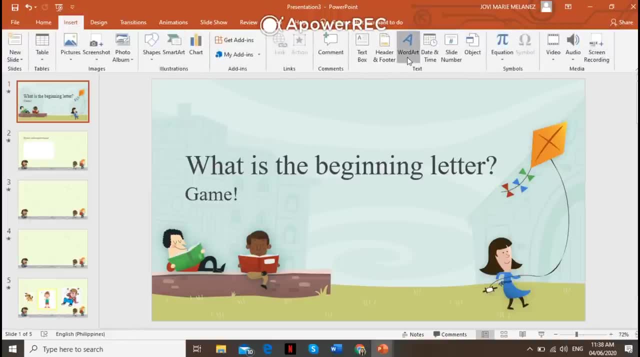 So let's make it simple, Because this is just a tutorial. What is the beginning letter game? So the first thing we're going to do here is to insert word art. So this is what we're going to choose. It's cute. 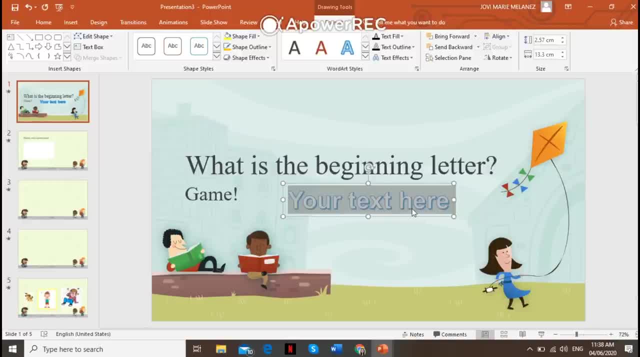 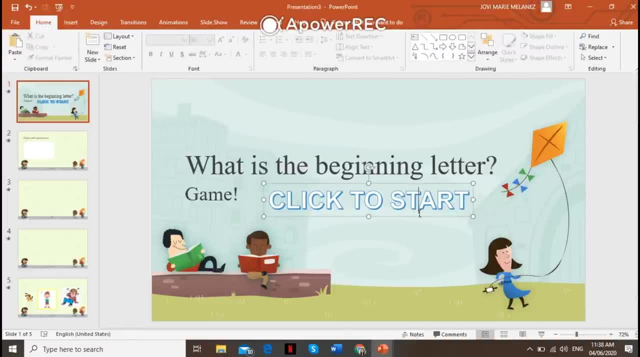 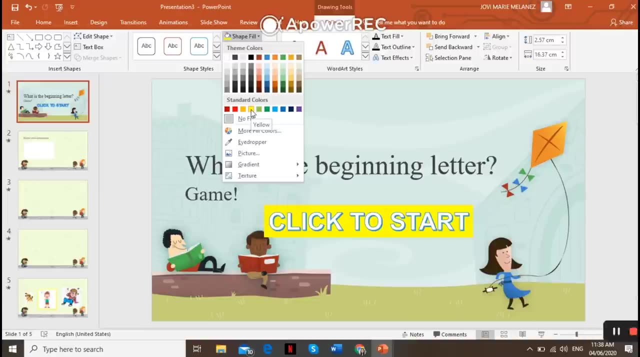 Click, And then we're going to put it here. Click to start. That is what they will click when they want to start the game. Let's just change the shape fill There, Then the shape outline. Okay, There. 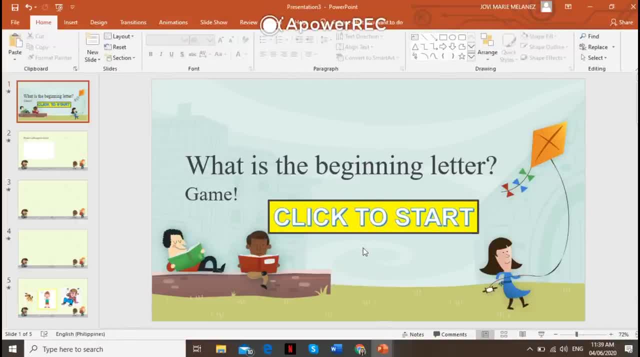 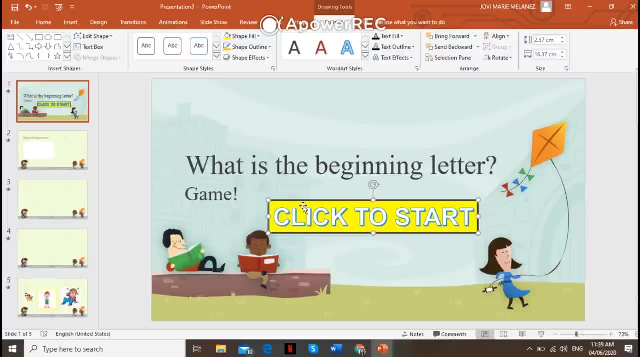 We can do that. So when we have that, let's go to the next slide. So what the kid is going to do when they listen to that? they will go straight to the next slide Or to the first item. 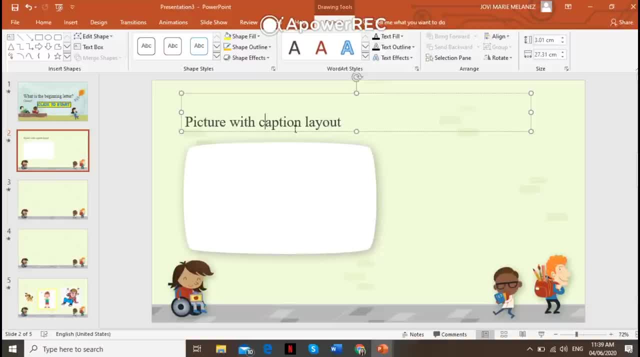 Okay, First item, Let's put the instruction: Click, Click on the letter or click on the beginning letter of the word that is in the box. So ito yung box natin. Then maglalagay tayo ng options dito. 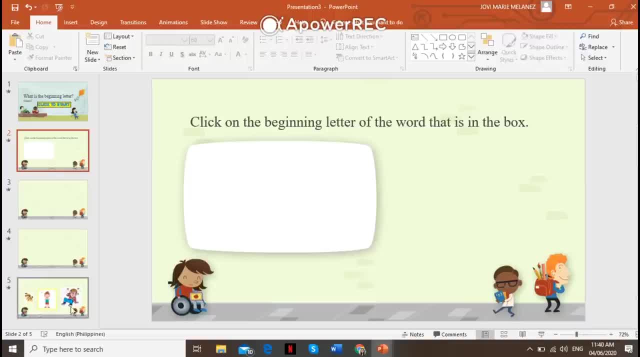 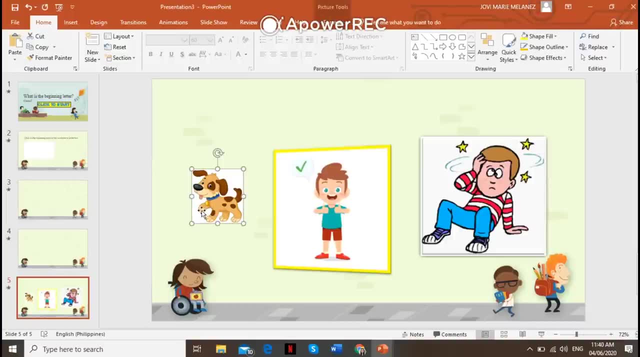 Dito nila i-click-click yung answers nila. So punta tayo sa fifth slide, Kung saan nilagay ko na yung pre-downloaded na pictures. Example: ang first item natin is dog. Click natin yan dyan. 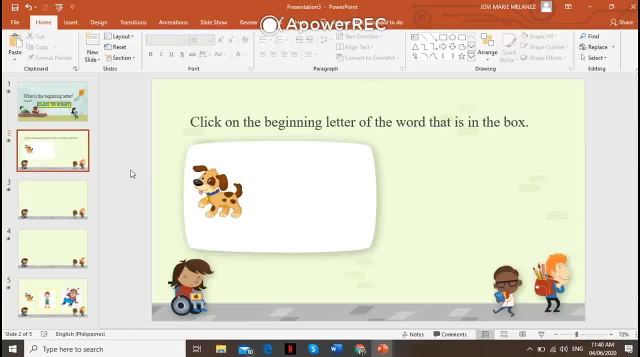 Ayan Dog. What is the beginning letter of the word dog? Kung mas bata ang mga client ninyo, pwede nyong ilagay yung mismong word dito na dog, para ima-match na lang nila yung beginning letter. 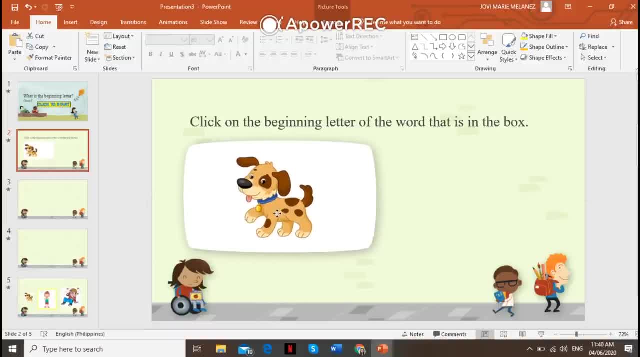 Pero dahil example naman, Pwede nating buuwin yan Example, grade 1, ang maglalaro nito, Pwedeng ganyan na yan, And then sila na lang ang bahala na mag-identify ng beginning letter. 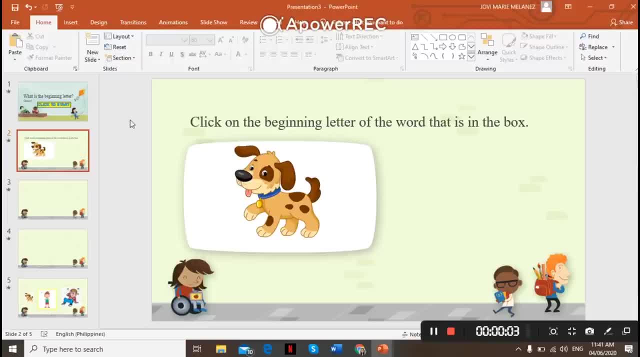 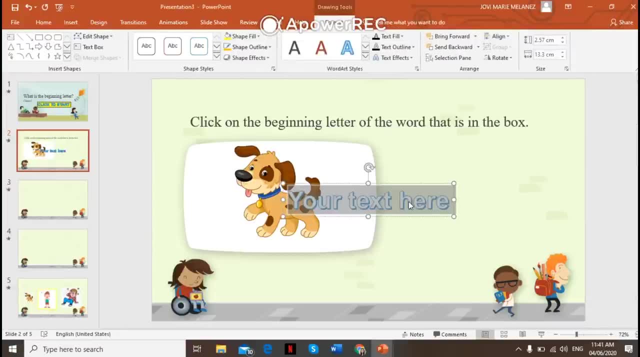 So after that, let's insert a text box or a word art- Word art na lang Ayan. And then let us put the choices: Letter D, Letter D. Then let's fill it with a color. Okay. 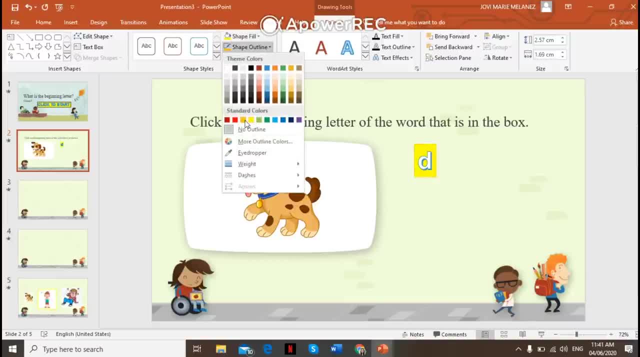 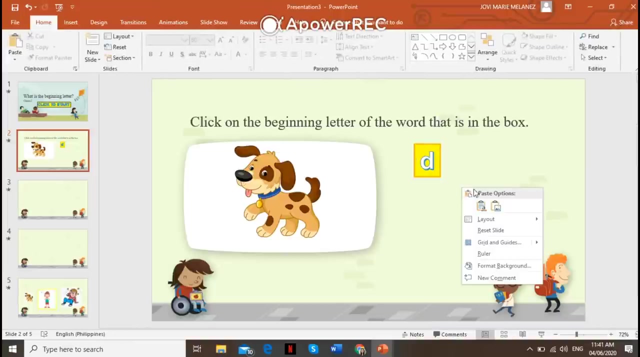 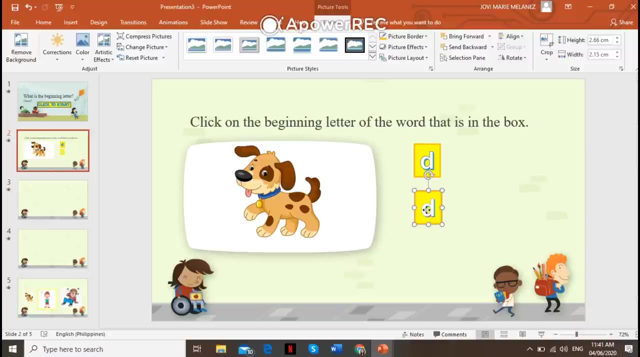 And then outline, Then yung weight ng outline Ayan, Para mas thick yung ano nya. After that pwede na natin i-copy and paste. Copy, Let's copy and paste Ayan. And then ang gagawin nyo na lang: i-change nyo yung letter sa loob. 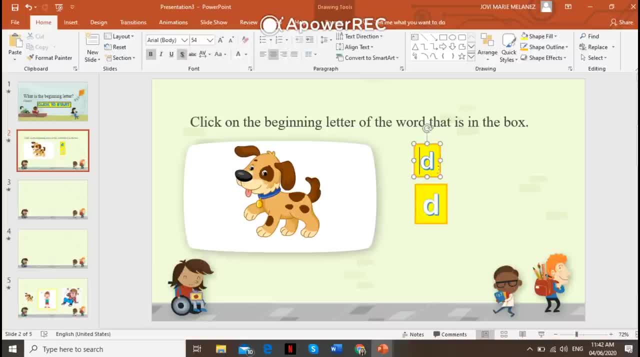 Ba't ayaw na. Ayan Letter E, kunwari Copy paste ulit. Then letter G, ang ilagay naman natin Copy paste ulit, Then letter R: Ayan yung choices nila. 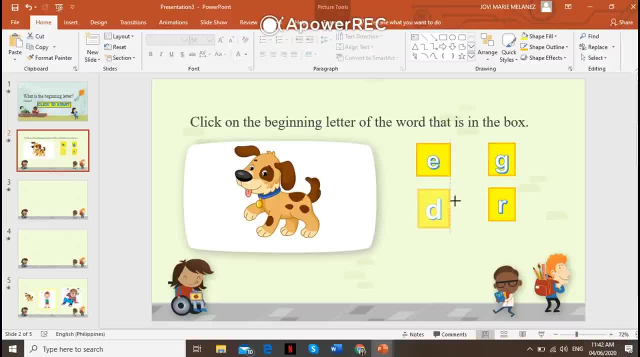 Okay, Lagyan natin diyan, Gawin nating pare-parehas yung size O kaya, lakihan na lang natin. Okay, That will do. We are now done with the first item. Nagawa na natin yan. 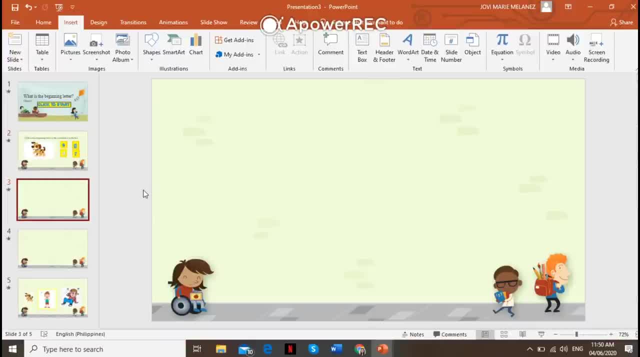 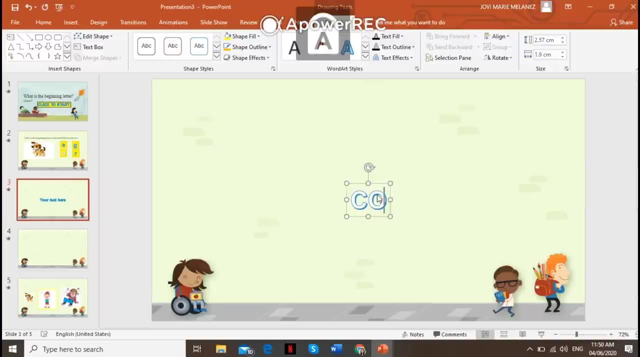 Now let's proceed to the third slide. Ang ilalagay natin dito is yung correct na answer or yung slide. Lagyan natin ng word art, Then ilalagay natin diyan, correct? 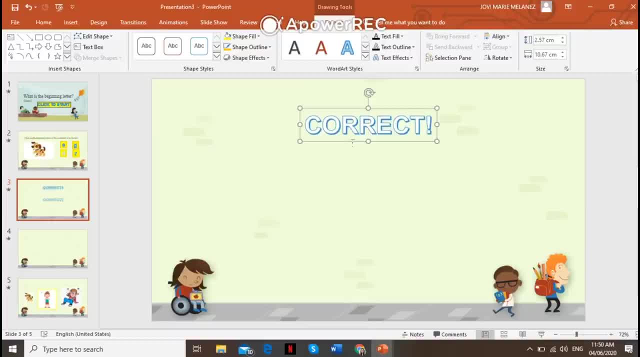 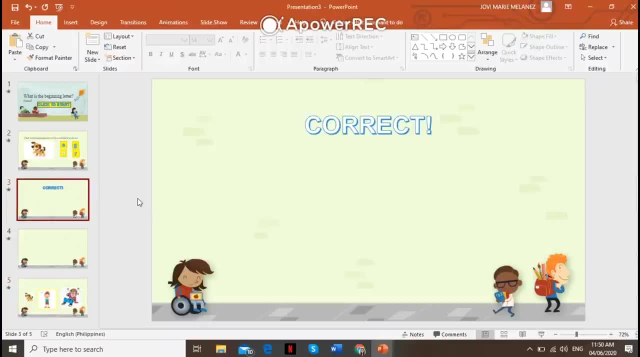 Ayan ang mag-a-appear kapag klinik ng bata yung correct answer. And then let's copy the picture na this one para mas maganda. Paste natin dito: Ayan, Ayan ang mag-a-appear. 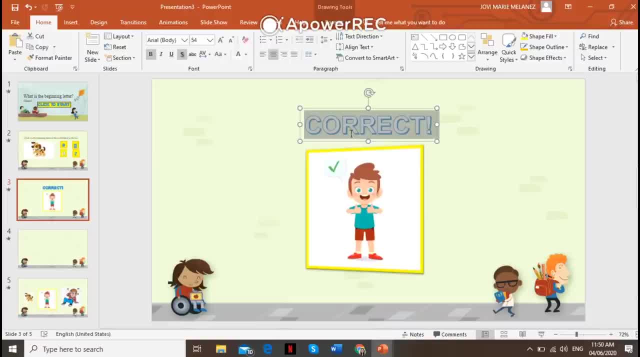 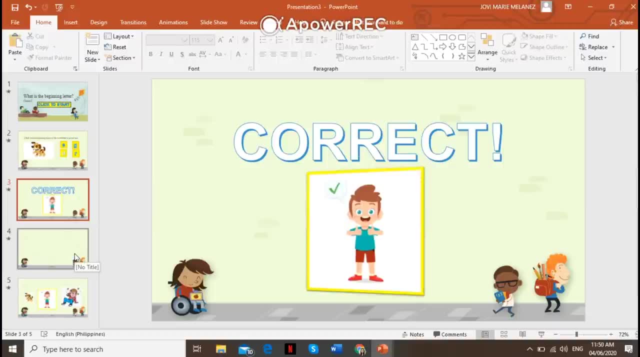 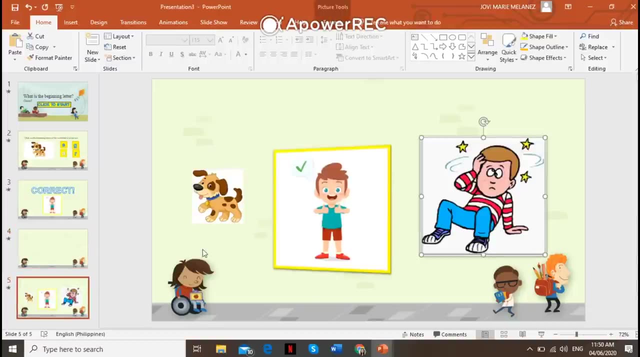 So let's proceed to Okay, lakihan muna natin yan Correct. And then let's proceed to the fourth slide. Ilalagay naman natin yung. try again the slide, Copy natin ito. 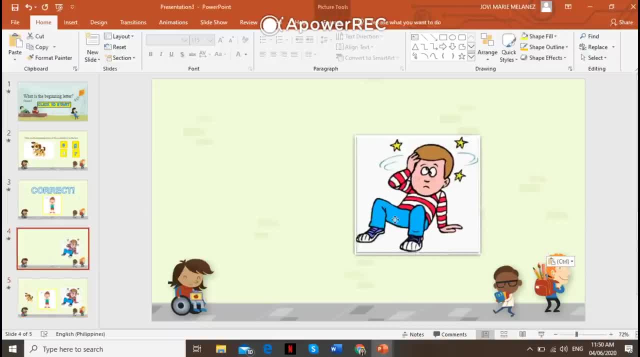 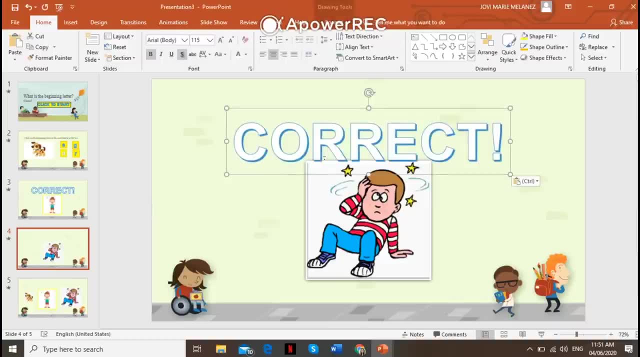 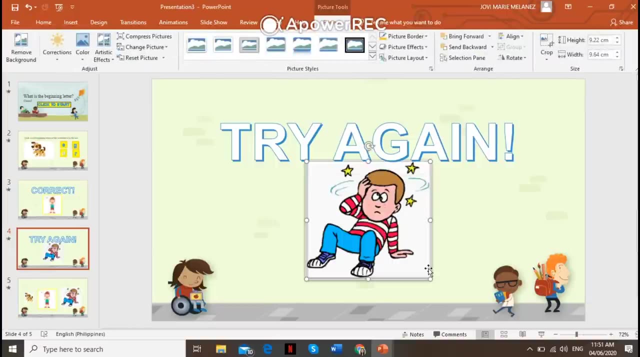 Then let's paste it here, Then let's copy this word art And then paste natin dito. Change natin yan ng try again. Encourage natin na kapag wrong yung answer, it's a try nila ulit. 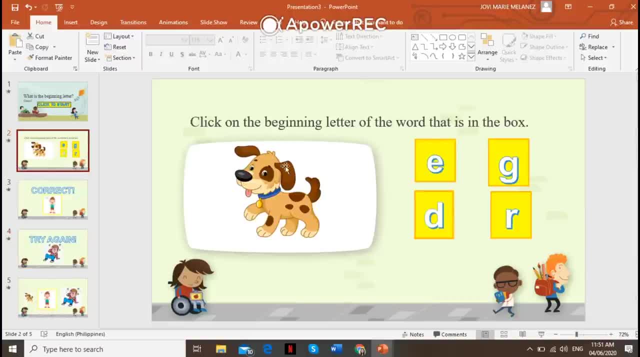 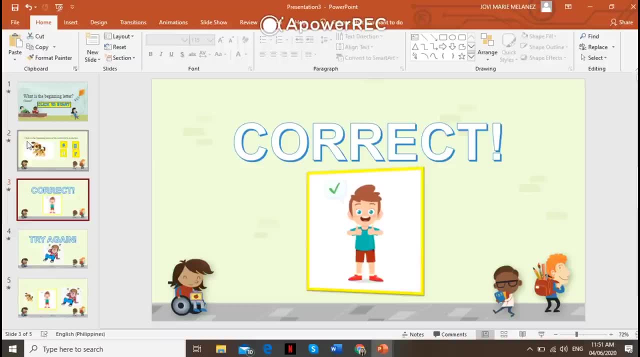 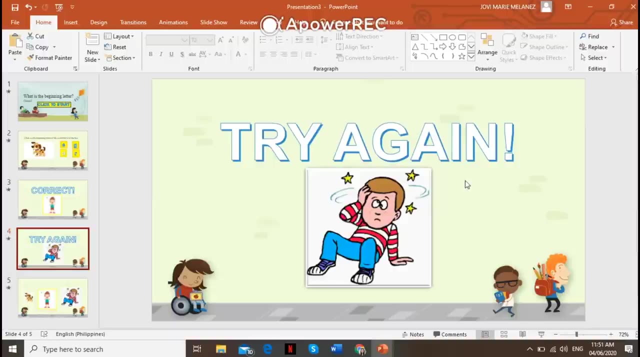 Right. So kapag pumunta dito yan nag-answer sila and klinik nila yan, automatic maglilink sa correct na slide. And then kapag klinik nila yung wrong na letter, automatic maglilink sa try again slide. 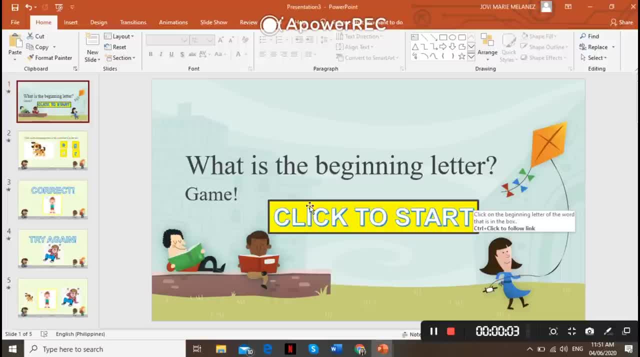 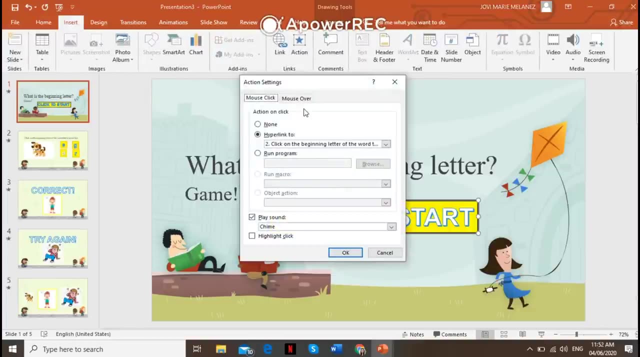 So let's try to put link na. First is: punta tayo sa title, Click natin ito, And then punta tayo sa insert. Punta tayo sa action, Click natin yan, And then punta tayo sa hyperlink 2.. 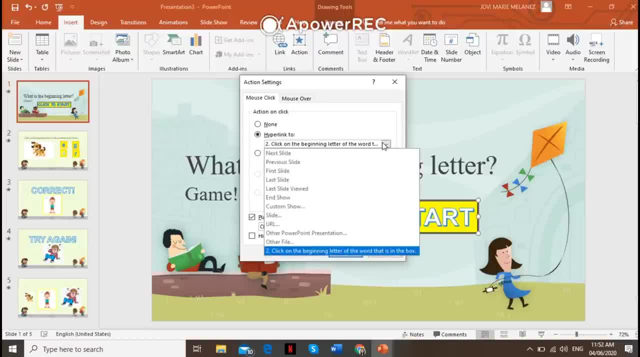 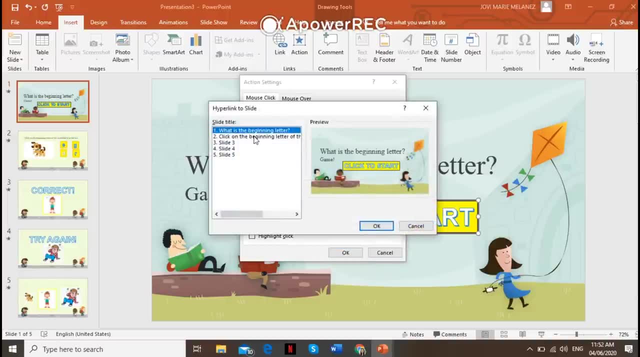 Click natin ito para may choice tayo And go to the slide, Click yung slide And then choose the slide na pag-proceedan ng option natin. So after clicking the click to start here, mag-proceed na yan sa first item. 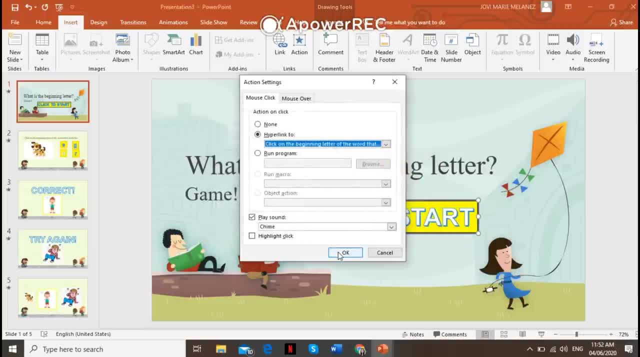 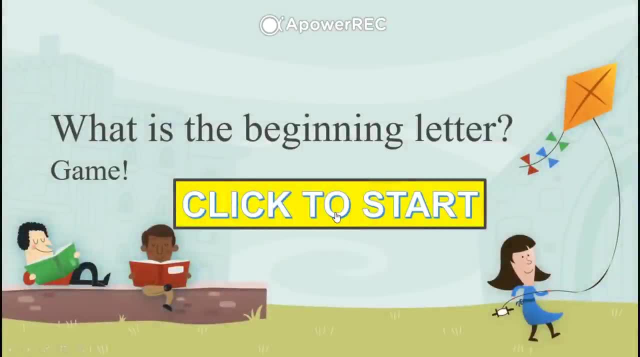 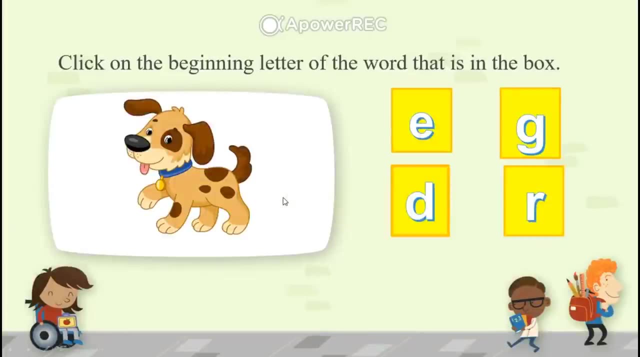 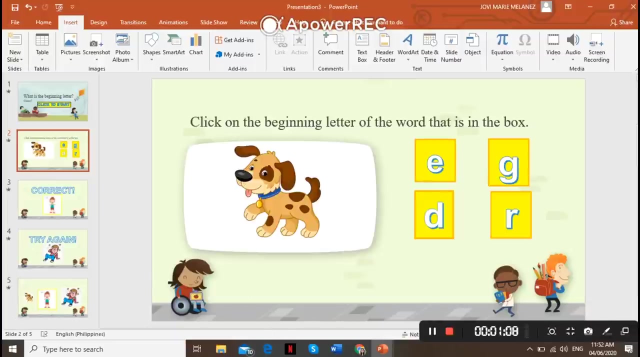 Click on the beginning letter. Yan, Okay, let's try, Let's try, So yan ang mag-a-appear. Then, if you try to click that, de-direksyo na yan sa first item. Okay, Next, lagyan natin ng link itong mga ito. 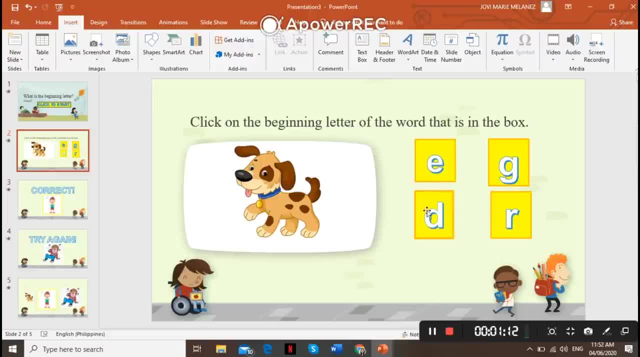 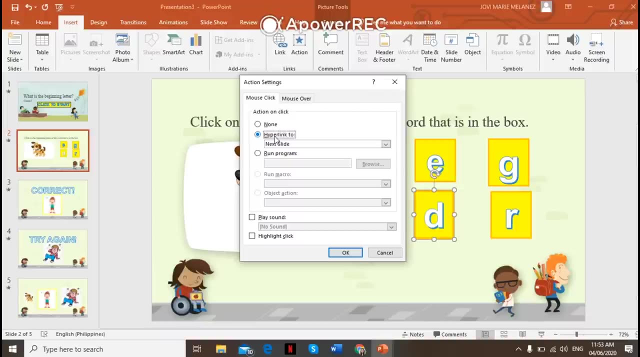 First yung correct answer. This is the correct answer, right Letter D. Okay, First lagyan natin ng link itong correct answer, Punta tayo sa insert, Then action, Click natin yung hyperlink 2.. 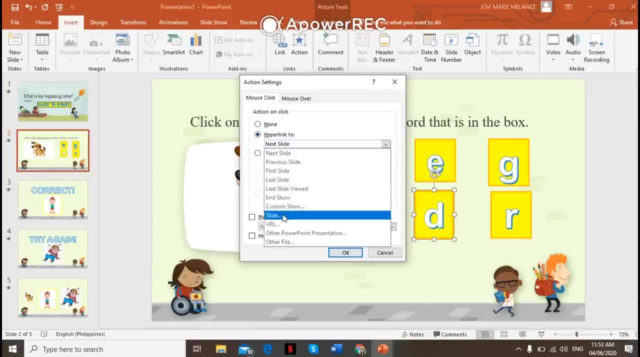 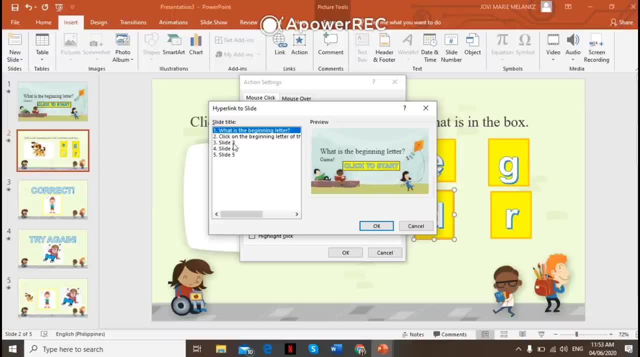 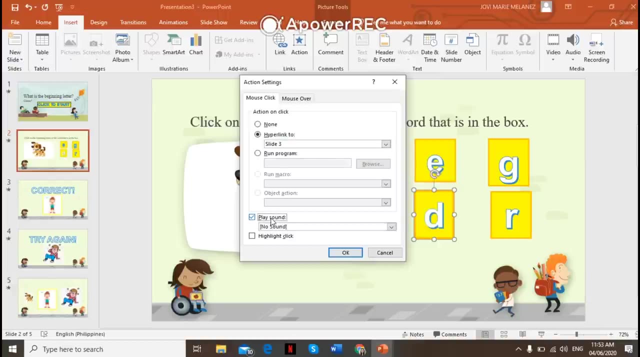 And then click natin ito, Go to the slide And choose the slide that you want to appear, Because it's the correct answer, yung slide 3, ang ilalagay natin Slide 3.. You can also put sound. 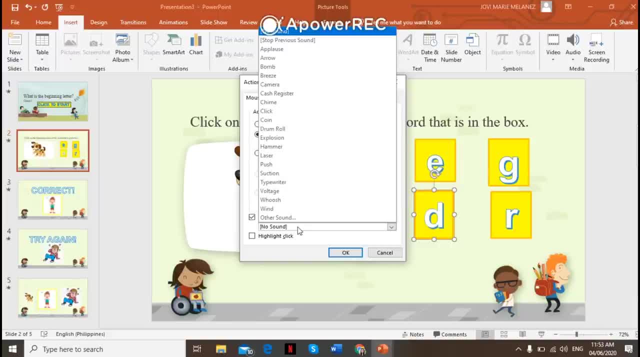 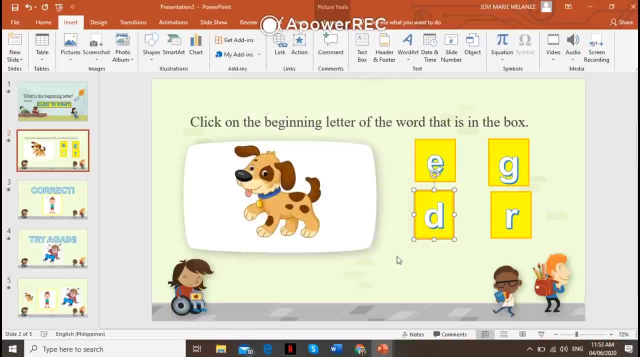 Play sound kapag linik nila yan. Dahil correct yung answer, ilalagay natin yung applause Right Once na klinik ng bata. ito ang de-direksyo is dito, De-direksyo yan dyan. 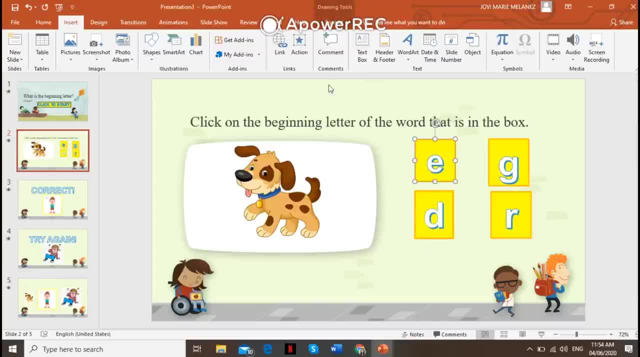 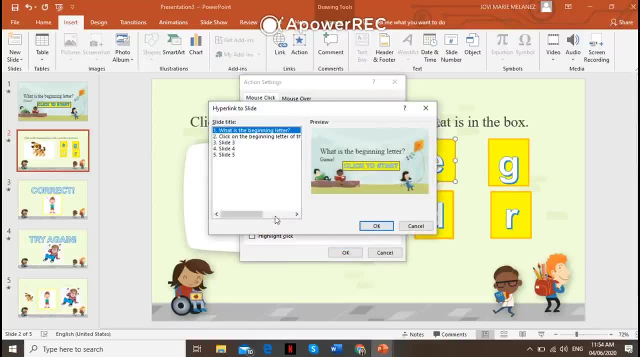 Pero kapag wrong yung answer, lagyan natin ng link. Punta tayo sa action Hyperlink 2.. And then sa slide. Doon tayo sa slide 4.. Dahil yun yung try again. 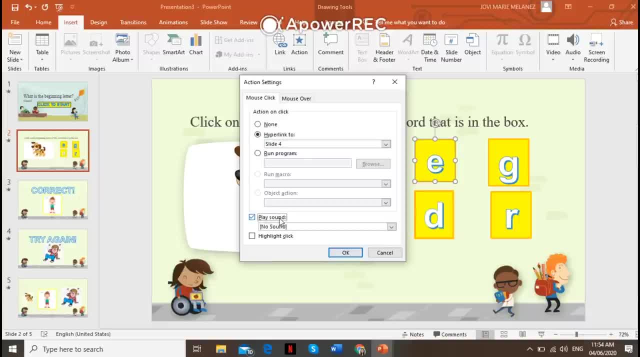 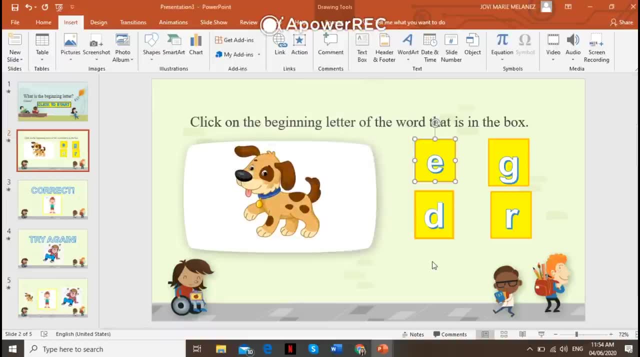 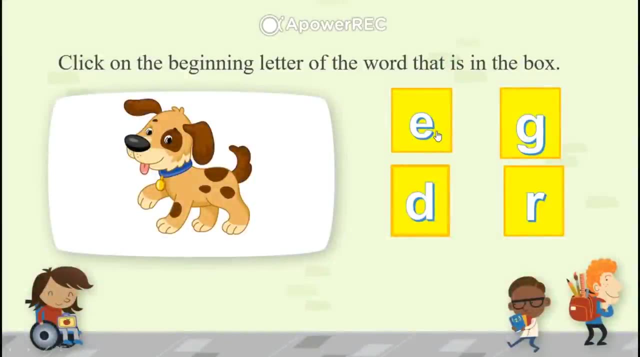 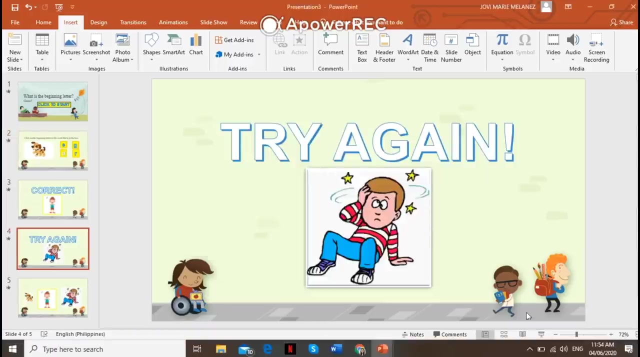 Right, And then let's put a sound. Lagyan natin yung whoosh. Okay, Let's try. Click natin yan. Kunwari, ito ang answer ko. Try again. Okay, Yun, yung mag-a-appear. 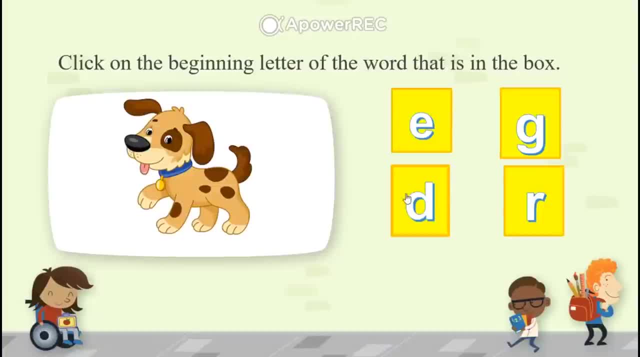 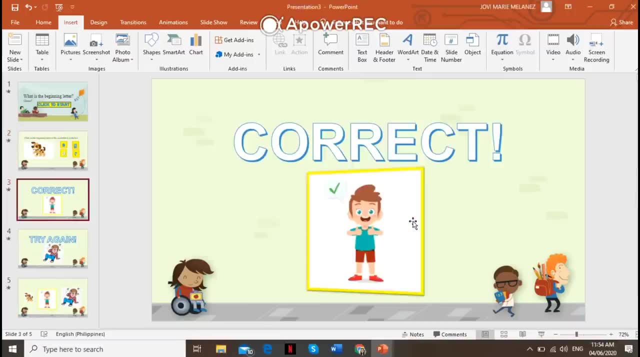 Now kunwari naman correct yung answer ko, Ito ang ikliklik ko Ito ang mag-a-appear. It's so easy, Diba, Kailangan lang natin gawin ay lagyan natin ng link ito. 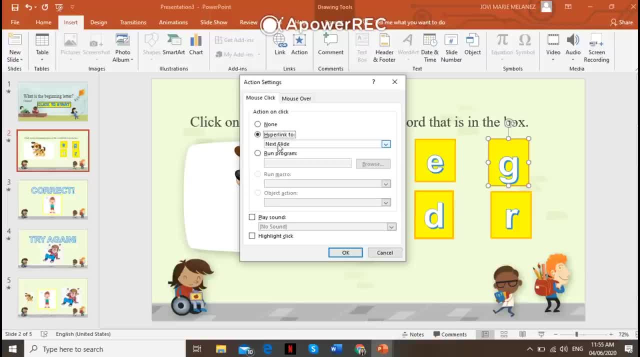 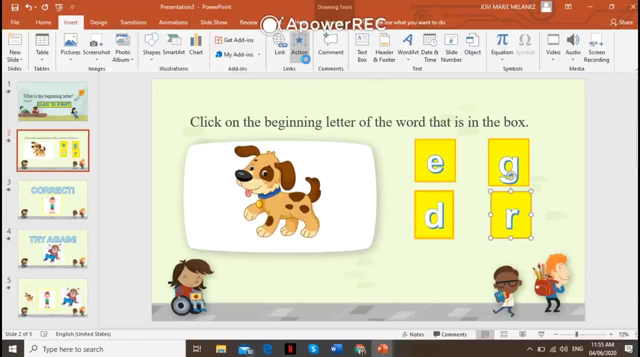 Sa action, Click sa action And then lagay sa slide na try again Slide 4.. Then lagyan natin ng sound Whoosh. Then same is true with the R. Wrong answer pa rin yan, Kaya, punta tayo sa hyperlink. 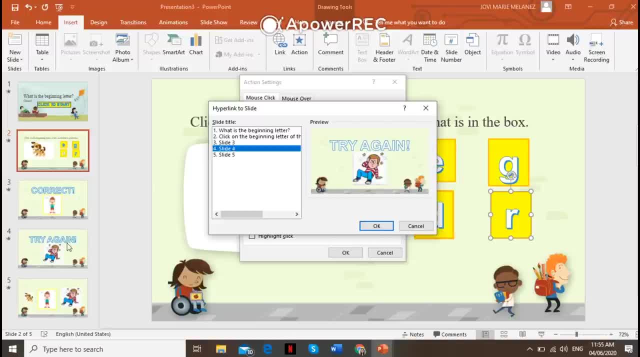 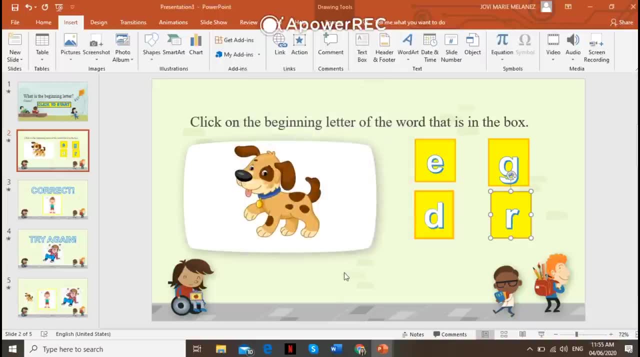 Tapos slide, Then slide 4.. Dahil yun ang try again. And then okay, Let's put sound Whoosh. Okay, Kapag tapos na to, Kapag nakuha na nila yung correct answer. 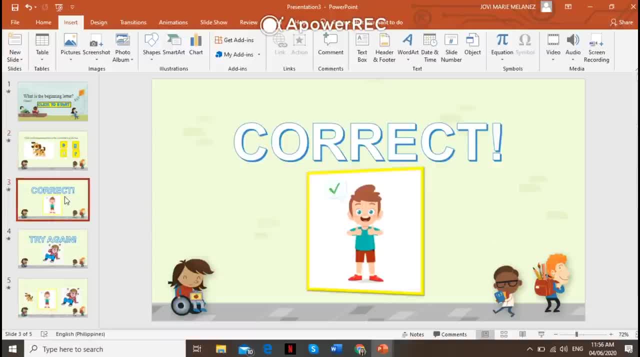 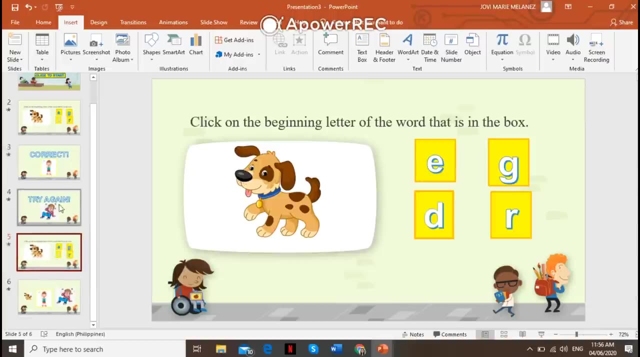 Example: clinic nila yung D At dederecho yan sa correct. Lagyan nyo ito ng hyperlink na naman Going to the next item. Example: ito yung next item. Duplicate natin yan, Then lagay natin dito. 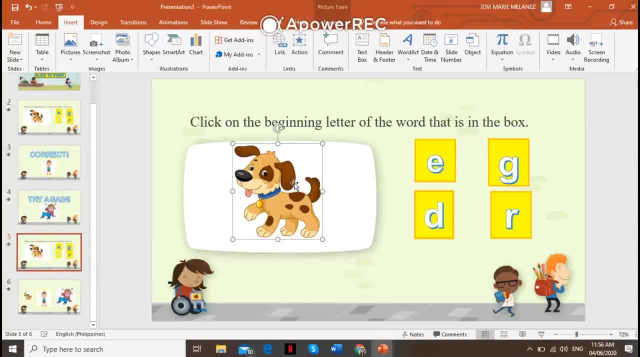 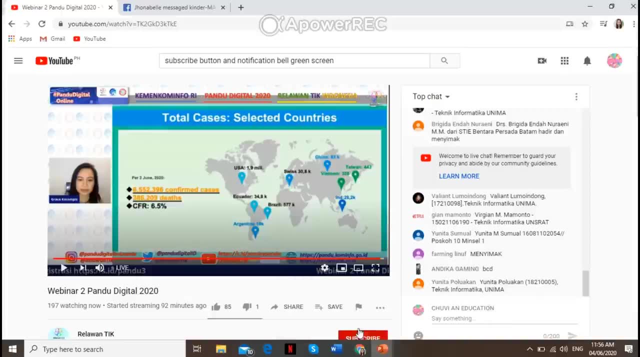 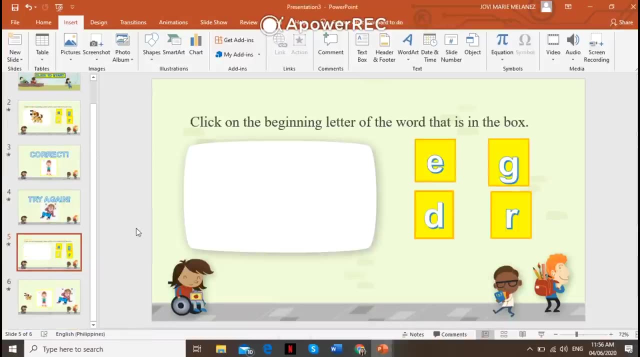 Example: this is the next item. Example: cat naman ito Cat. Okay, Delete natin yan. Okay, Where are you, Cat? Let's copy this one. Yung ginawa ko na original, Ilagay natin dito. 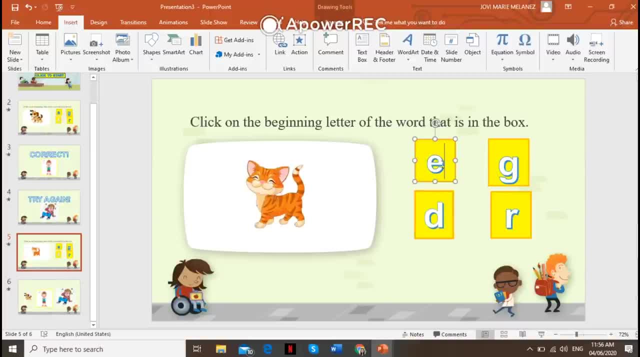 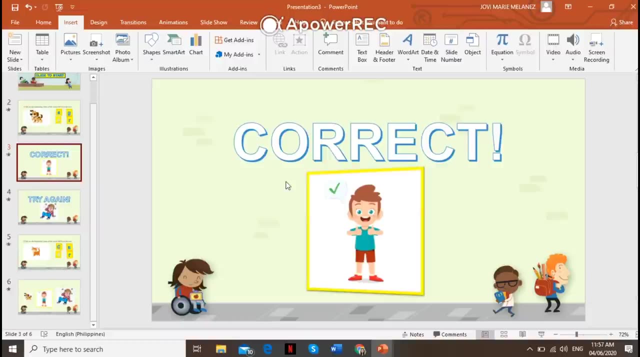 And then change natin ito Into C, Parang yung ginawa ko kanina. So balik tayo dito. Kapag clinic nila yung D Dederecho yan sa correct Ibig sabihin. 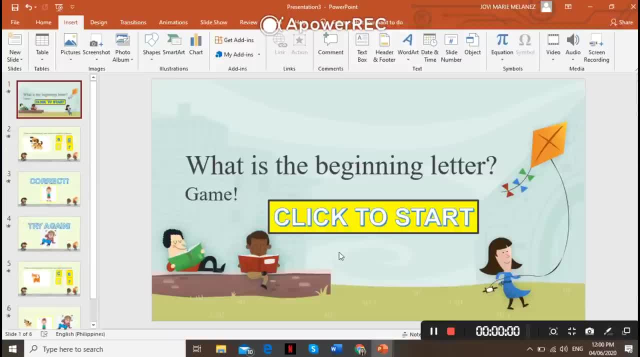 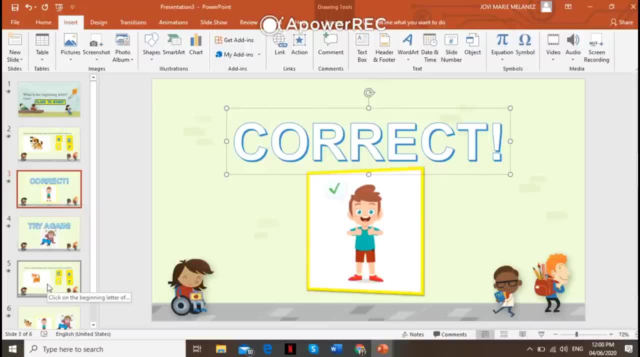 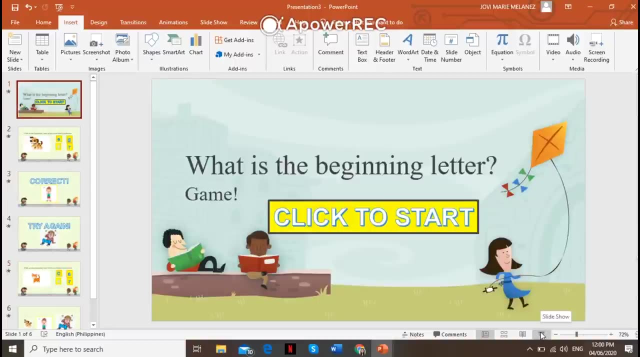 Ibig sabihin pwede na silang mag-proceed sa nila Right Kapag clinic nila yung correct, Dederecho na yan sa next item. So let's start. Let's start the game, Try natin. 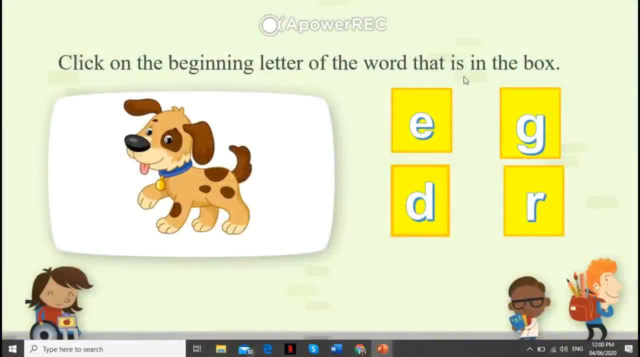 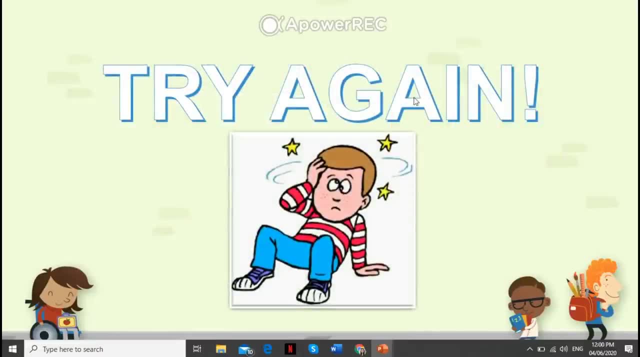 Click to start. Click on the beginning letter of the word that is in the box. So what is this? It's a dog Kunwari. wrong yung answer ko. Okay, Try again. Kailangan natin itong lagyan ng link para babalik yan sa. 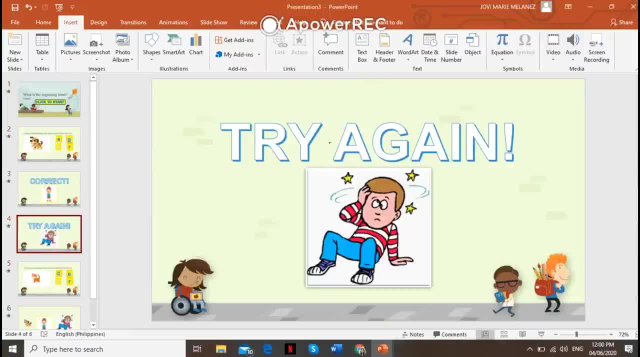 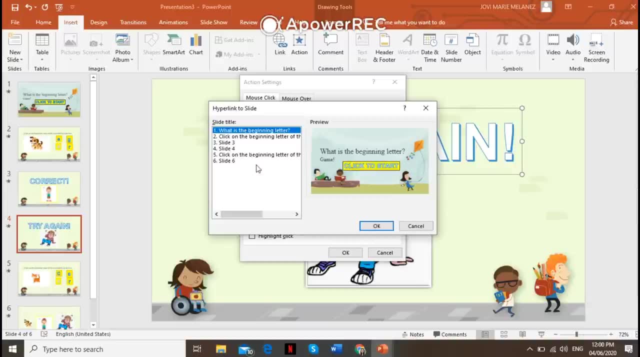 Babalik yan dito. Okay, Lagyan natin ng link, Ito Hyperlink, Then punta sa slide, Then slide number 2.. Kasi nga wrong yung answer, So try mo ulit. 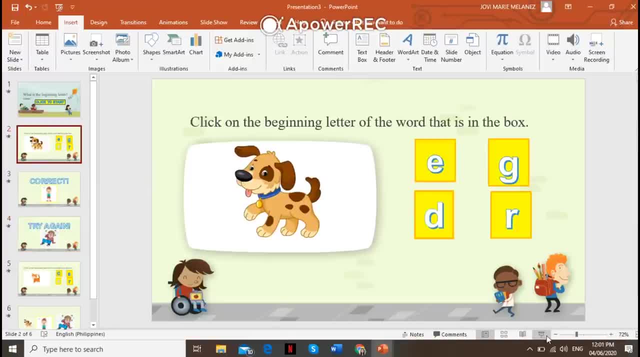 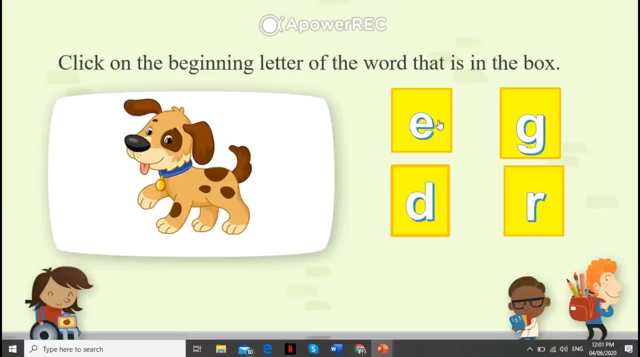 Okay, Ulit natin Wrong yung answer ko Kaya Wrong yung answer ko Kaya ilalagay O dyan O try again. Then balik ako. Click Yan Itatry ko ulit.